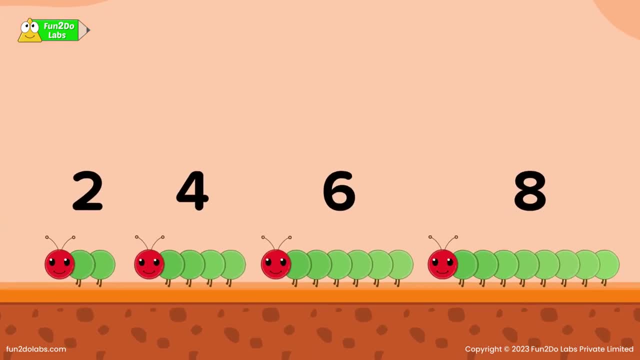 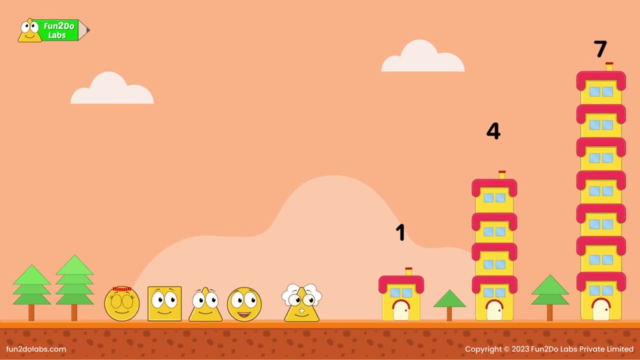 Yes, their bodies are also increasing by two. Look at those beautiful buildings: One floor, four floors and seven floors. Wow, The floors of the building are growing by three. Now do you get how things grow differently on Growing Pattern Land? Yes, Uncle Math. 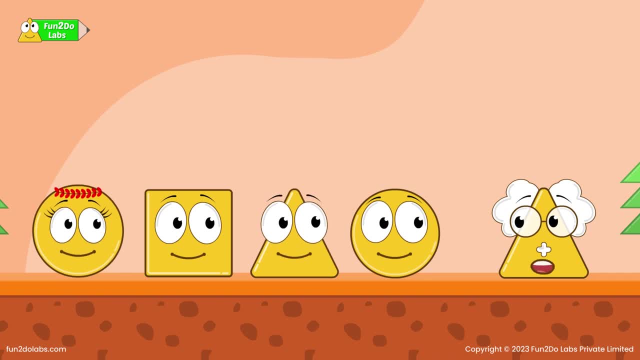 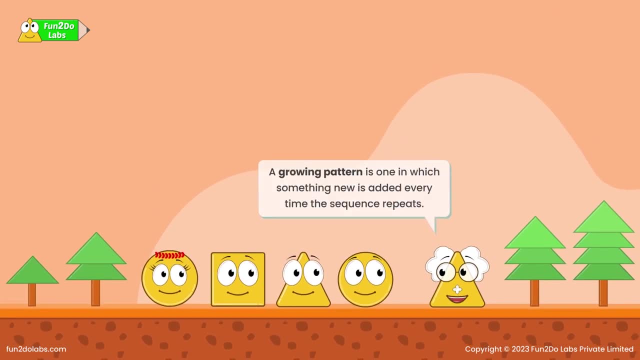 Everything here is growing in size. They are growing in a pattern. Such patterns are called Growing Patterns. A Growing Pattern is one in which something new is added every time. the sequence repeats, Like in trees. every time a new layer was added. In caterpillars, two new body circles were added. 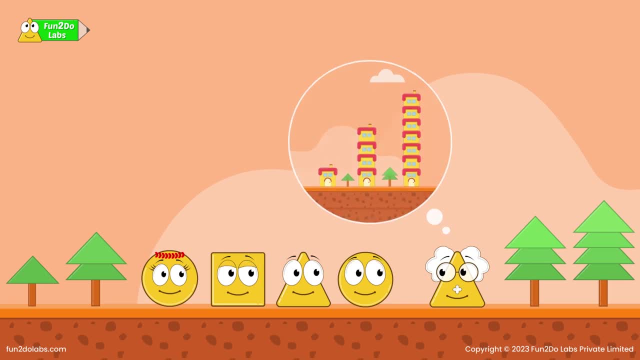 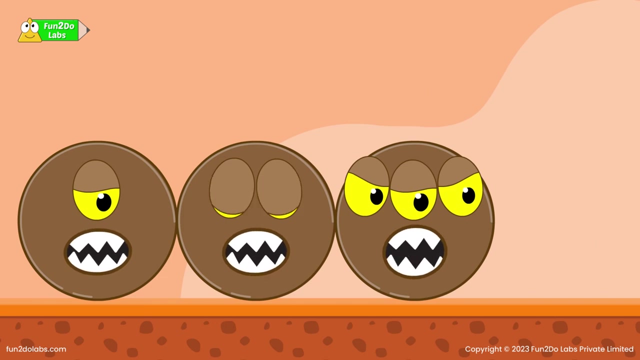 And finally, in buildings. every time three new floors were added, They hear the sound of heavy steps. suddenly, Slowly, the sound gets louder And the ground starts vibrating too. What is happening? Oh no, The growing monster. Suddenly, there appears a growing monster whose eyes are growing in numbers. 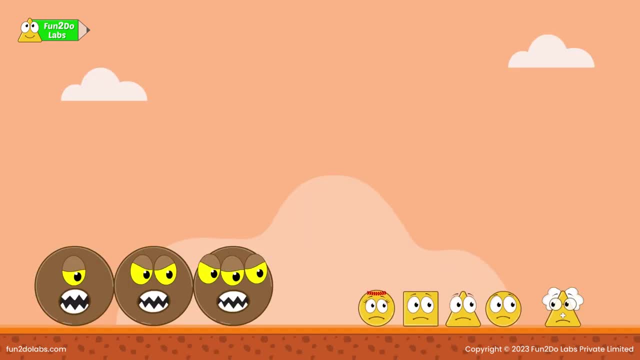 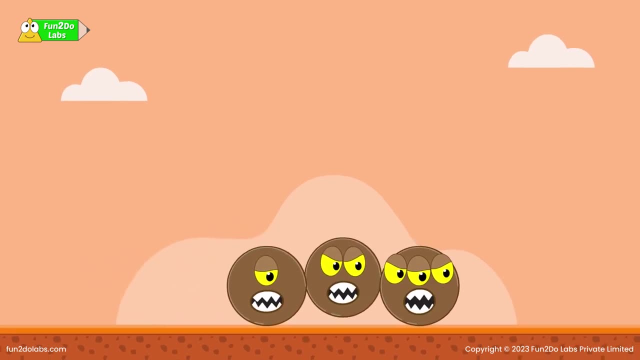 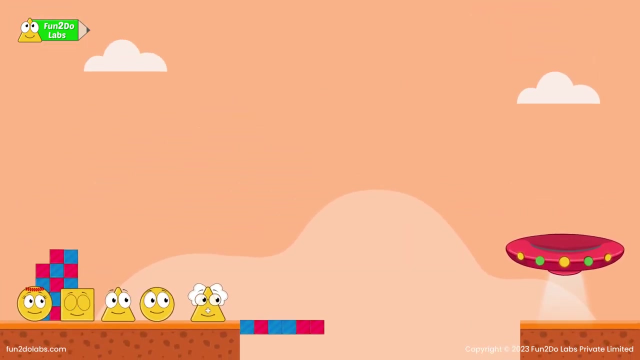 So scary He will eat all of us. Uncle Math guides everyone to run towards the spacecraft. The scary monster follows them Soon they spot their prey. Uncle Math tells them to run towards the spacecraft at a distance. But there is a problem. 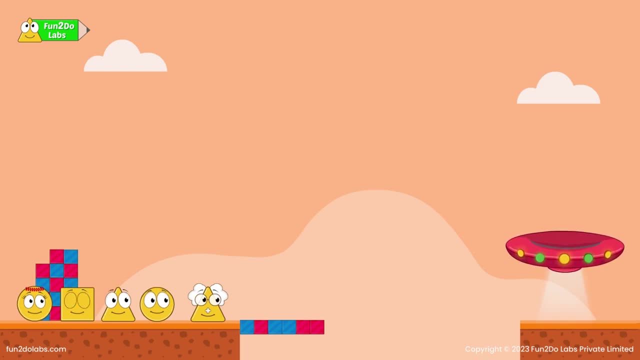 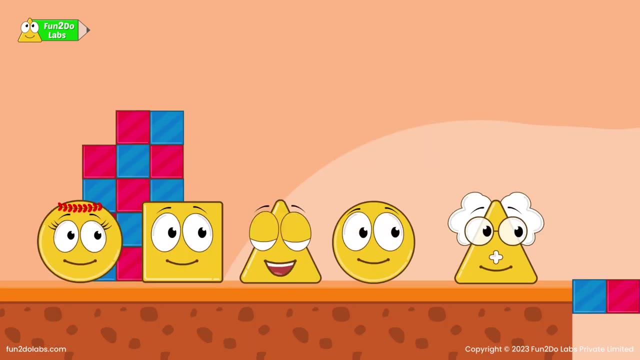 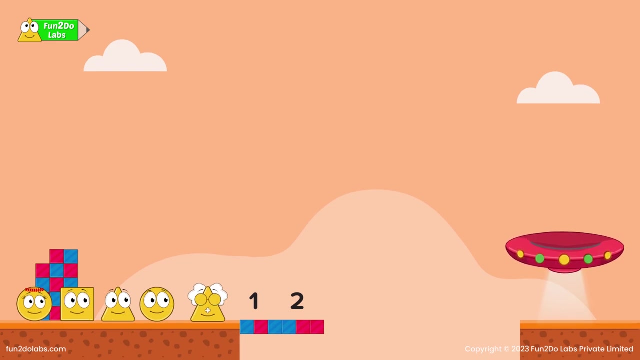 The bridge leading to the spacecraft is incomplete, But the monster is very close. What can they do to save themselves? The bridge also has a growing pattern. See the blocks are increasing by one, following the order of blue and red blocks. Let us quickly complete the bridge following the same growing pattern. 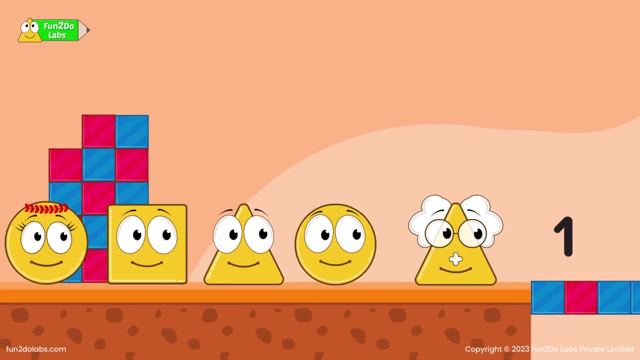 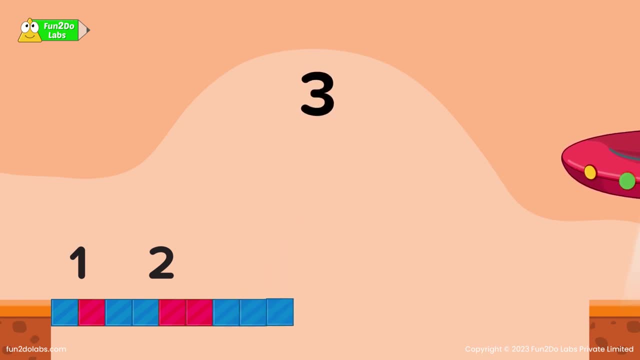 Yes, let's complete the pattern Together. they start building the bridge using the blocks. They start with adding three blue blocks, then three red blocks, Unable to reach the spacecraft, yet they continue. Can you guess how they add the blocks to complete the bridge? 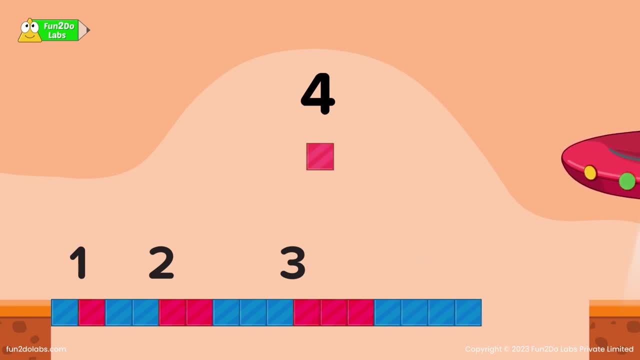 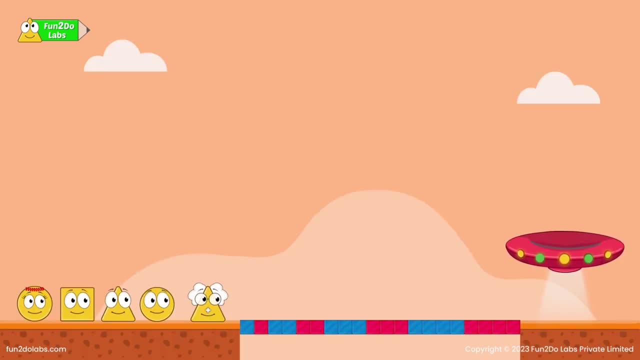 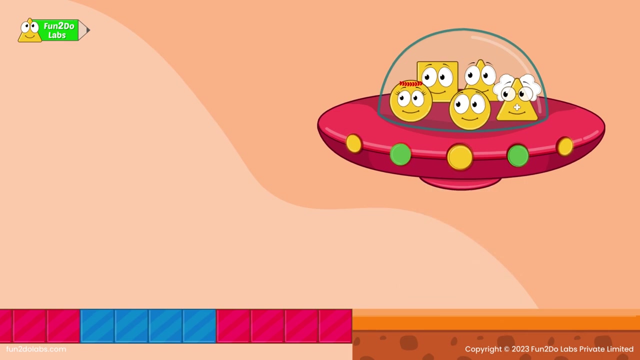 They added four more blue blocks and four more red blocks to complete the growing pattern on the bridge. Finally, they are able to complete the bridge Run Run. They swiftly reach the spacecraft and board it. Uncle Math flies it as quickly as he can.